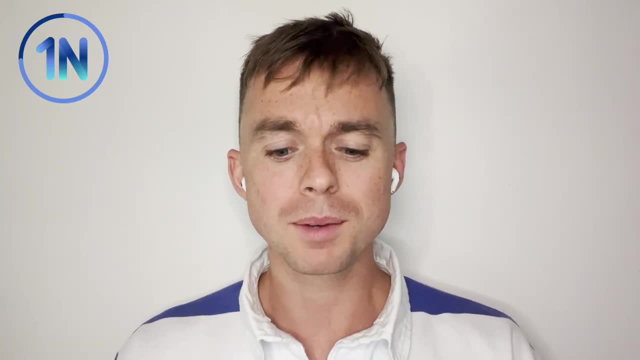 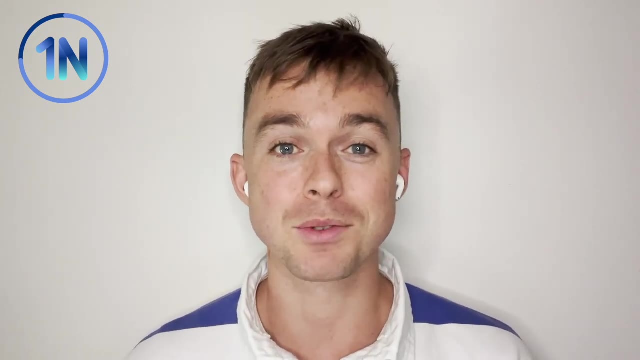 just as much as we need, but we're going to put this together. You're welcome to try and build this view using Sample Superstore. That's totally cool If you want to save yourself some time. you just want to get straight to the practice. why not download this? It's in the 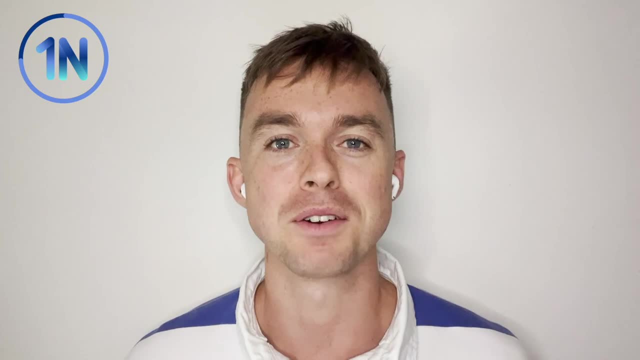 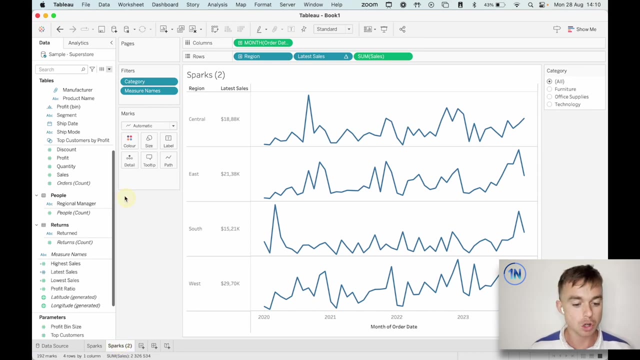 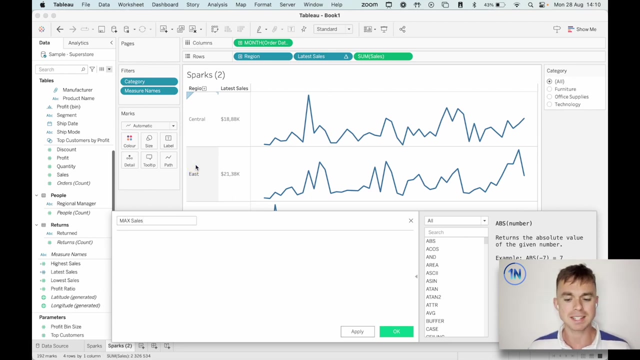 description below on my Tableau Public, and then you can just fire it open and follow along as we go. Okay, let's dive into it. So I'm going to navigate to this worksheet called Sparks 2 and I'm going to create a field called Max Sales and I'm going to say something like this: 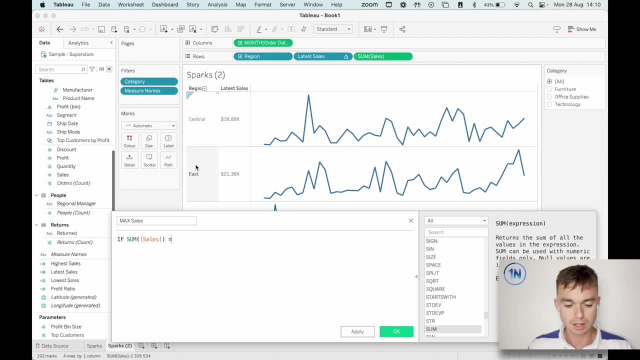 If the sum of sales is less than or equal to the sum of sales, then the sum of sales is less than or equal to the window max. sum of sales, then sum of sales. So what do we ask Tableau to do? Well, we've just. 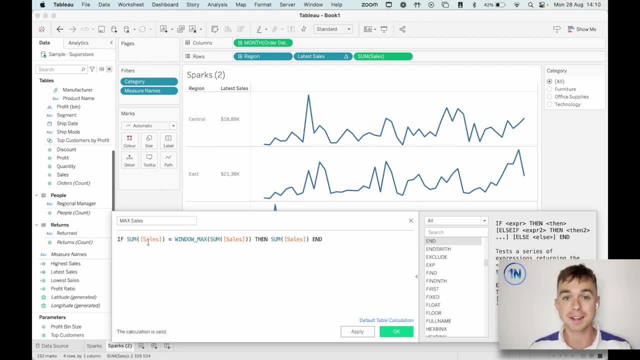 said: hey, if any of these sum of sales values that you encounter are the same as the maximum sum of sales value in the window, then return that sum of sales value. right, That's all we've said. So search through all the data in the window. return the maximum sum of sales value in the window. 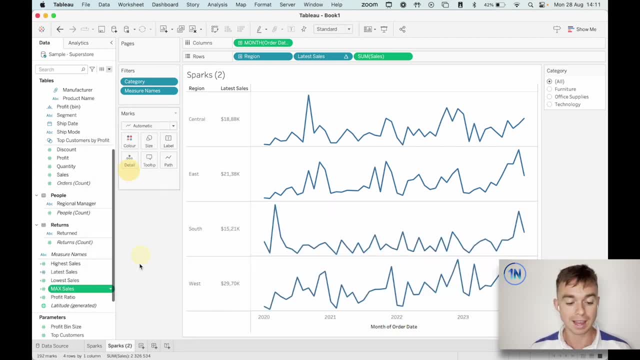 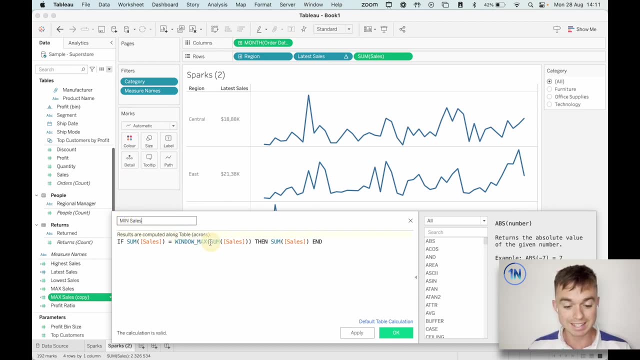 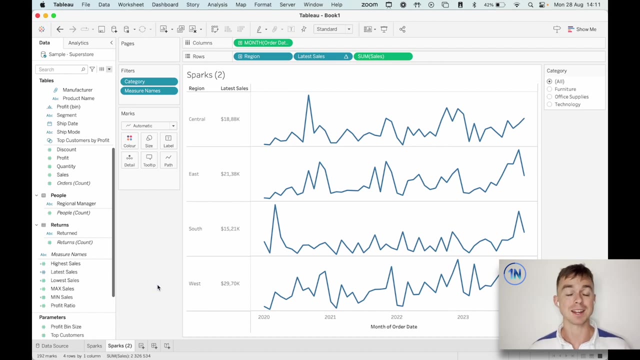 let's hit. OK, We can just duplicate this, because now we need a min sales value and the logic is exactly the same, except we change max to min and we're good to go. Okay, so we're going to put this all together and help to isolate those values, But let me just say that, if this is interesting, 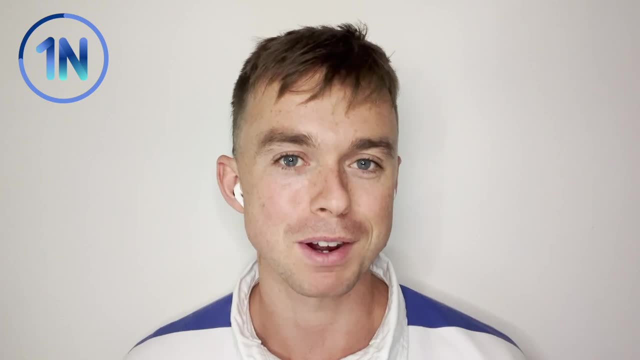 to you and you want to learn more about Tableau, why not join us for one of our courses? We've got some super cool courses coming up If you're interested in learning more about Tableau. we've got some super cool courses coming up, all the way from Tableau- beginner courses to Tableau. 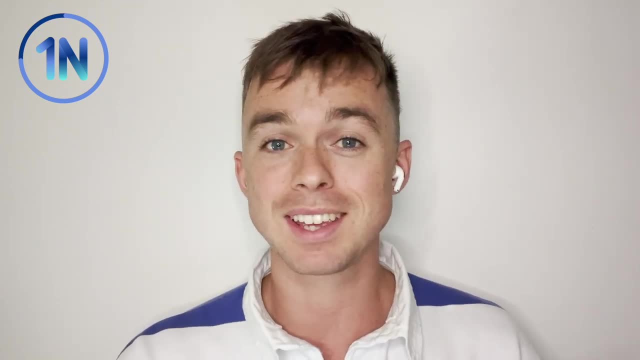 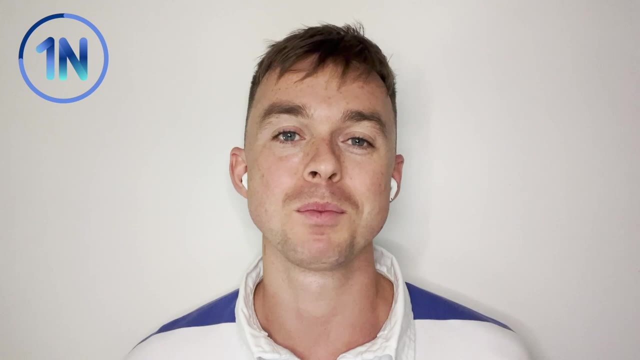 advanced courses, Courses focused in on just calculations and Tableau all the way through the Tableau prep. So we'd love to see you there. That would be super fun, And if you need any more help with your Tableau stuff, why not grab an office hour and we'd be so happy to help? Awesome. 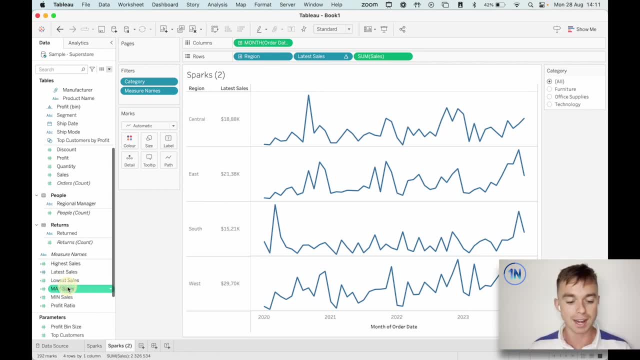 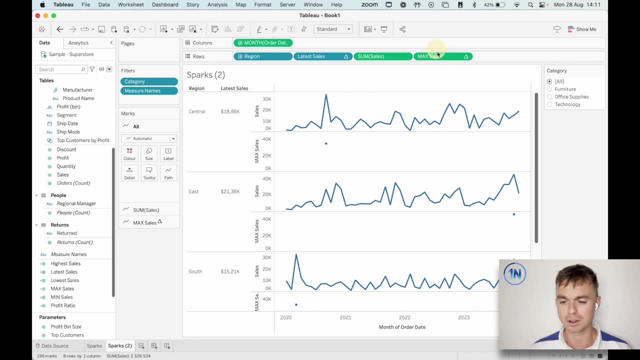 So let's do this. Here's how we're going to put this all together. I'm going to drag max sales up here onto the rows shelf. So Tableau has generated its, you know, kind of this weird graph for max sales. It's just a point. It's technically a line graph. 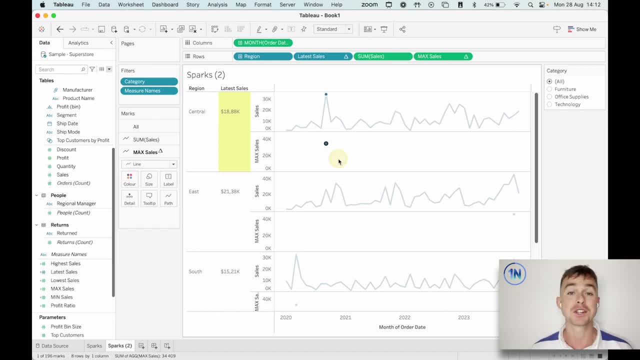 right. Tableau's automatic one was line, but it's just one point. Why? Because we've said the max sales needs to sum of sales, needs to equal the max sales and then return that sales value. That's exactly what Tableau has done. But here is the magic: We're going to drag this min. 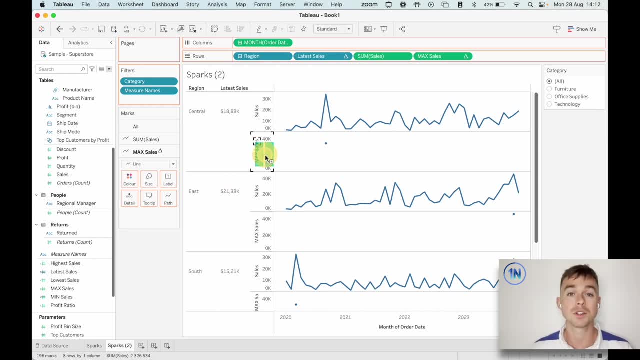 sales over here, So over the axis, when it creates those two. you know green bars side by side. maybe you've made a side by side bar chart before. it's the same technique and we're just going to drop it in And what that's going to do is Tableau has changed our 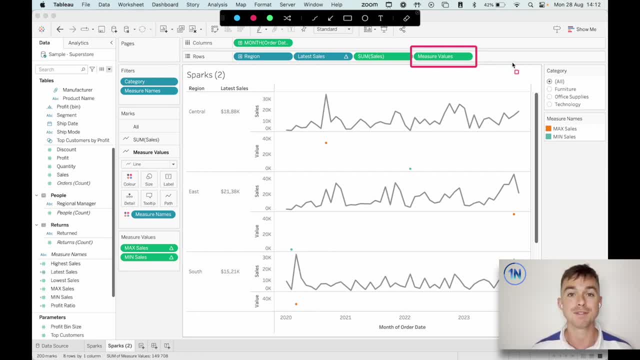 max sales value on the rows shelf to measure values. Now measure values. just a quick reminder. it's just a placeholder for multiple measures that might be in your view. In our case, this measure values pill now contains the max sales and min sales values. 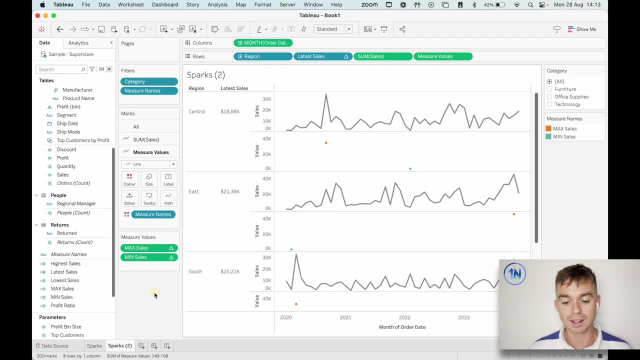 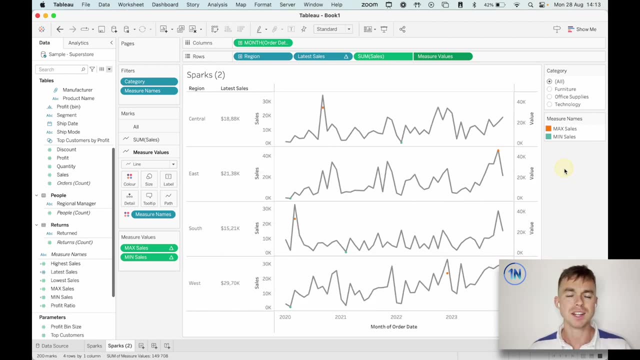 which is awesome. And the reason why this is such a win is that now we can right click on our measure values pill and say dual axis. So technically we've dual accessed three different measures right. We've created a dual axis chart out of min sales and max sales and sum of sales. 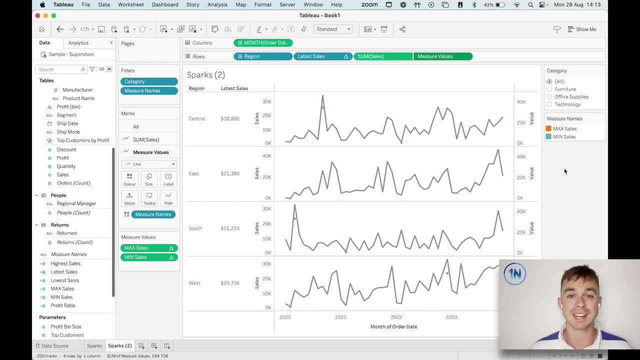 which is amazing. So that's just a helpful tip slash trick for your Tableau development in general, But for this view it's also super useful. Now, for those of you who are used to dual axis charts, you'll know- probably the first thing- that- 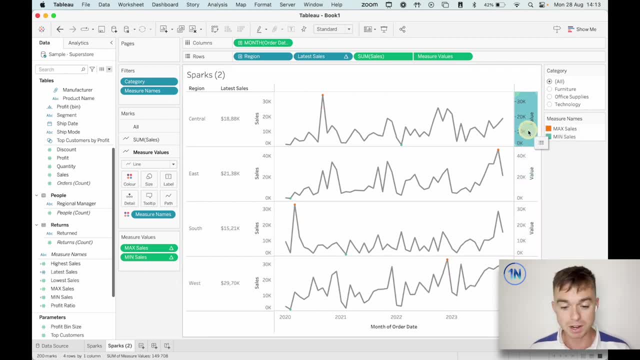 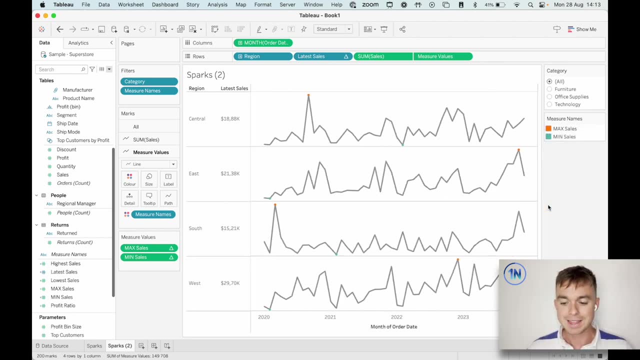 you're checking is: do I need to synchronize this axis? Yes, we do, So let's synchronize it and then uncheck show header. We don't need the headers for this example. Then the last couple of formatting tweaks that I'm going to do is I'm going to change this line under measure values to circle. 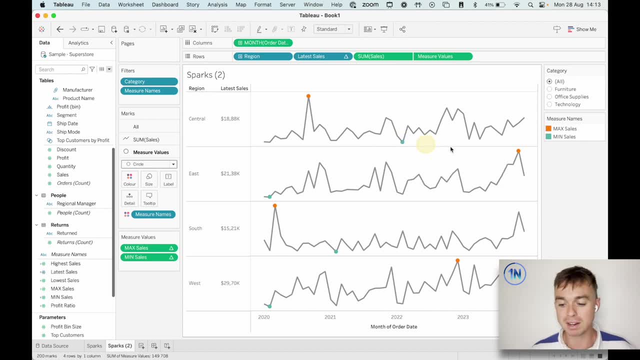 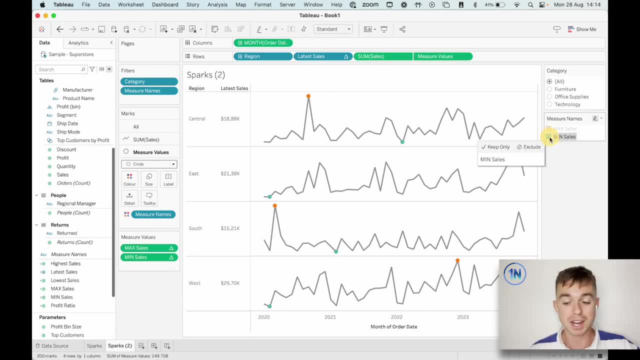 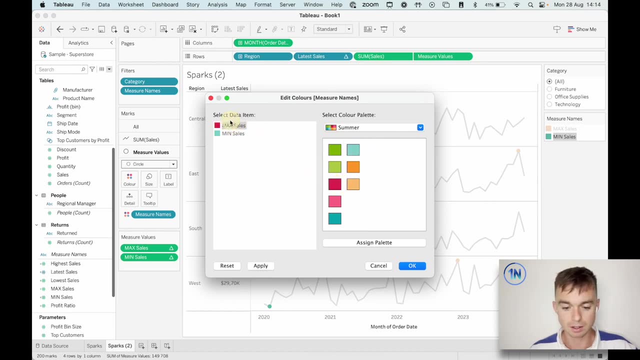 The colors. if we want to actually like those colors, that's quite nice, But if we wanted to change them, you just double click, choose a color palette that you like and, you know, get some of these going. We should probably do this the other way. Min sales and max sales.